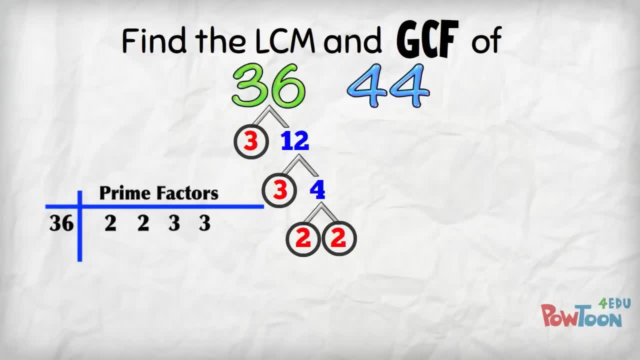 2 x 2 x 3 x 3. Clear the area 44 is from 4 x 11. 4 is from 2 x 2. Put those prime factors into the table, aligning like factors: 2 x 2 x 11. 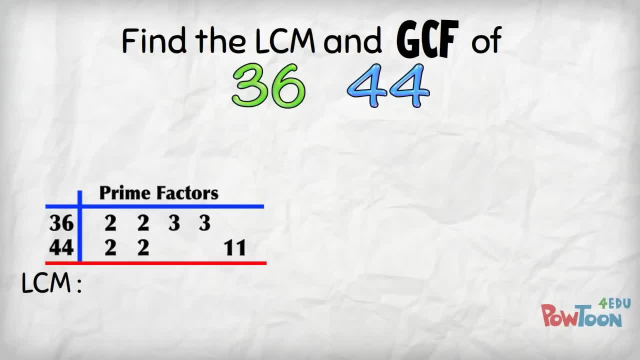 Now get the factors of our mystery LCM: 2 x 2 x 3 x 3 x 11. Work it out: 2 x 2 is 4 x 3 is 12 x 3 is 36 x 11. 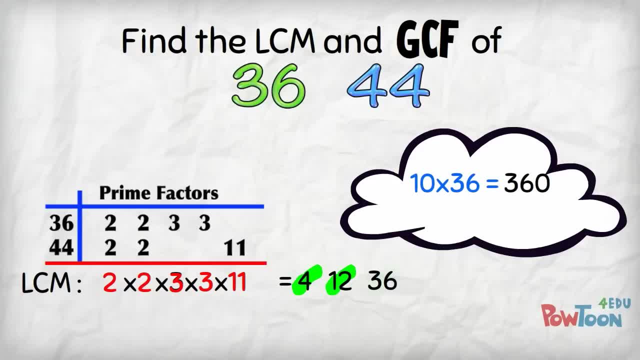 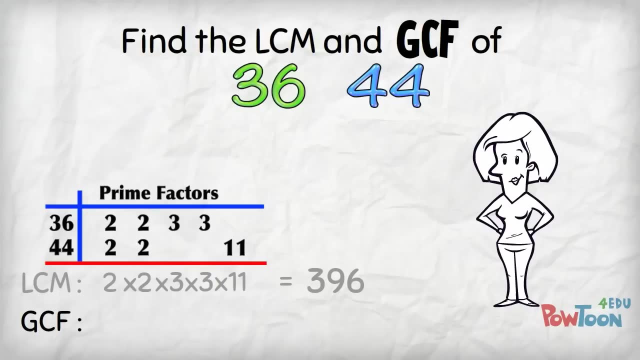 10 x 36 is 360. and add another 36 on that makes 11 x 36: 396. That's our LCM. Now let's do the greatest common factor. If a prime factor is common to both the numbers listed, then it is used in our greatest common factor. 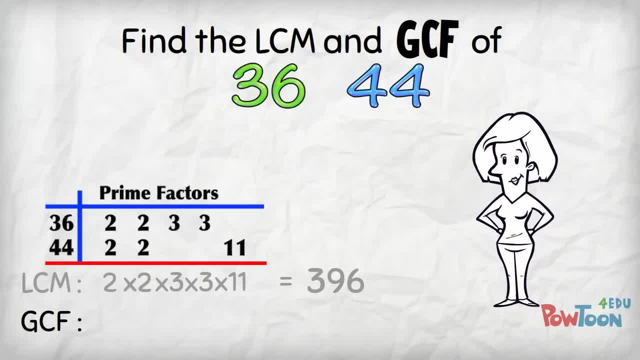 2 is in both lists of prime factors. Here and here. 3 is not common, nor is 11. List the common factors 2 and 2.. Then we multiply the common prime factors to get the GCF, So 2 x 2. 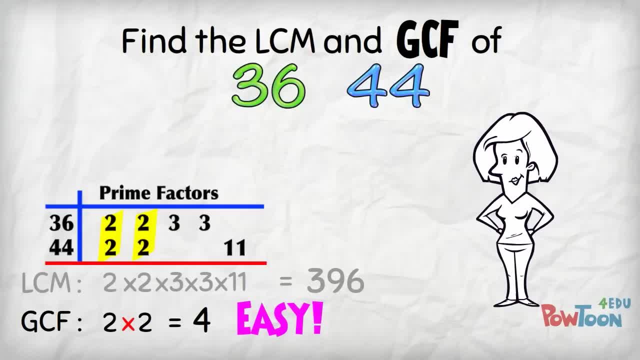 The GCF is 4.. Isn't that easy. I think it's beautifully simple and it's really fast after doing the LCM. If you use the prime factors, table 2- to help organise yourself as you're working through, you're going to find it very clear. 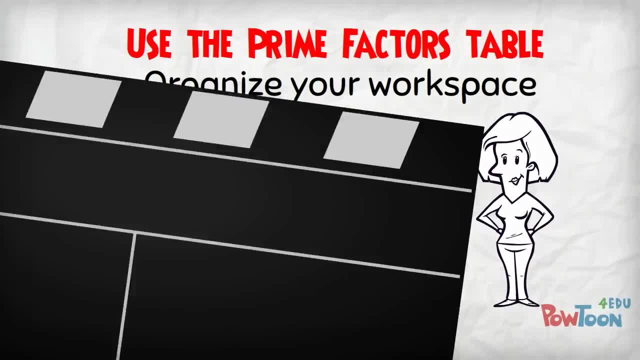 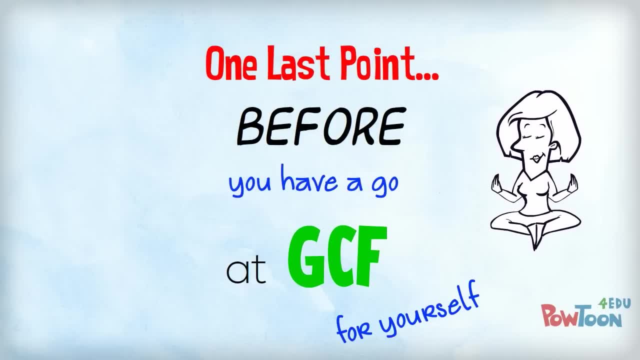 and you'll be least likely to make a mistake. There's one last point you need to be aware of before you have a go at GCF for yourself. At some point, your teacher is going to give you a pair of numbers, a bit like this: 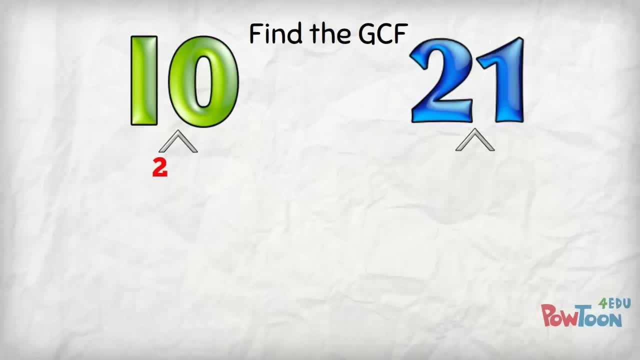 where, when you do the prime factorisation, you find that there are no prime factors that are common to the two numbers. So how do we list the GCF? If there are no factors common to the two numbers, then the GCF, the greatest common factor, is 1..